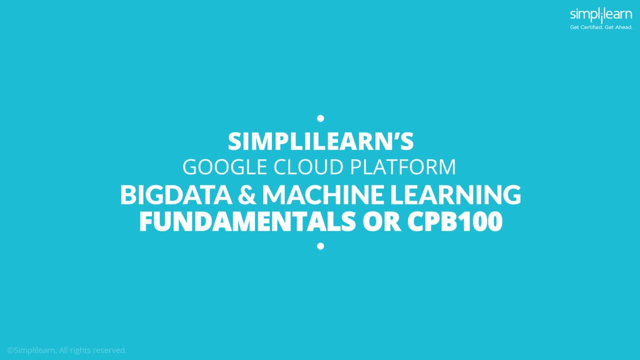 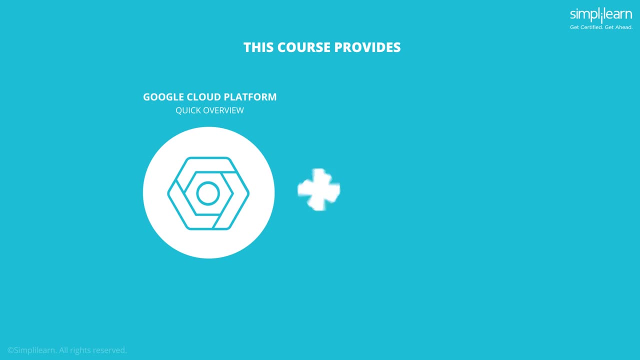 learn more about your business, how to manage your data and how to make better use of the data. SimplyLearn's Google Cloud Platform- Big Data and Machine Learning Fundamentals, or CPV100, offers a thorough overview of the Google Cloud Platform, covering its data processing capabilities. 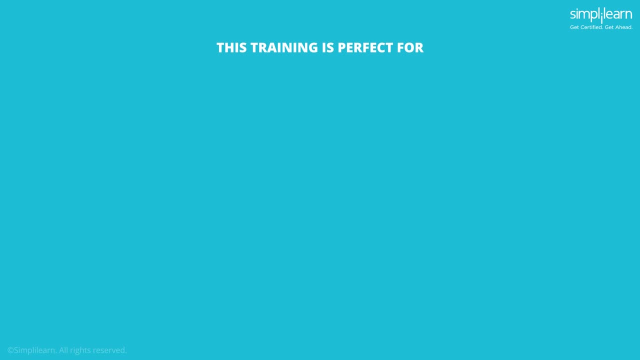 with various use case studies. It's the perfect course for data analysts, business analysts and business engineers. You can use it to be a Google's data analyst and even a business analyst and data scientists with real-world experience in querying, ETL, data modeling or machine learning. 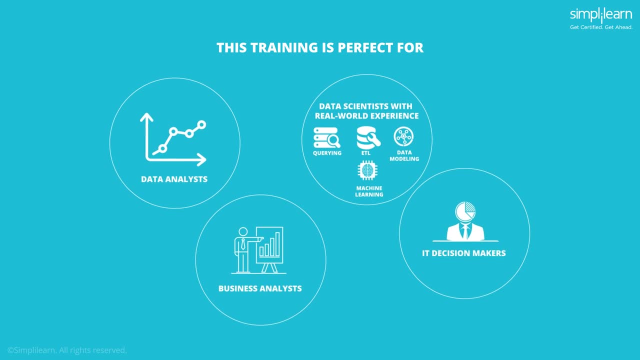 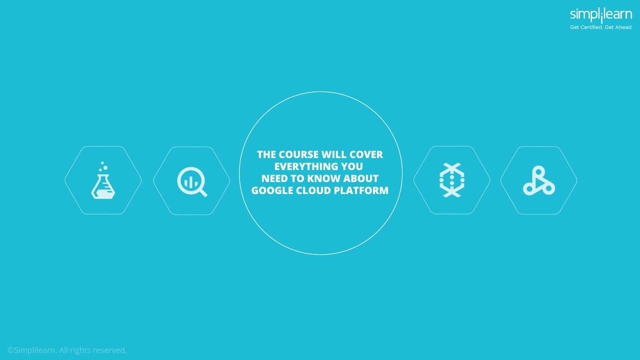 IT decision makers evaluating the Google Cloud Platform have also found the training very useful. The course will cover everything you need to know about the Google Cloud Platform and includes 8 hours of instructor-led training modules on big data and machine learning with the Google Cloud. 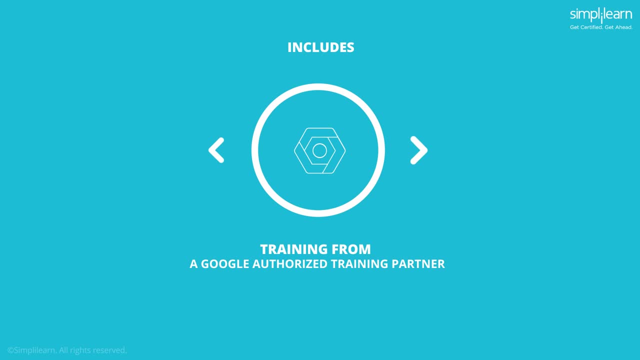 training from a Google-authorized training partner: 7 hands-on live lab exercises to reinforce your learning. So what are you waiting for? Register now and start learning. 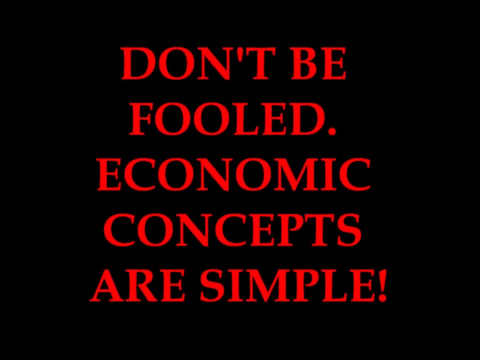 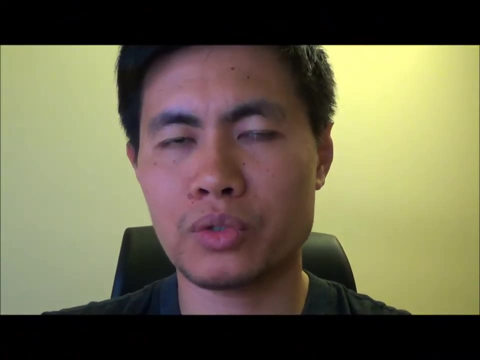 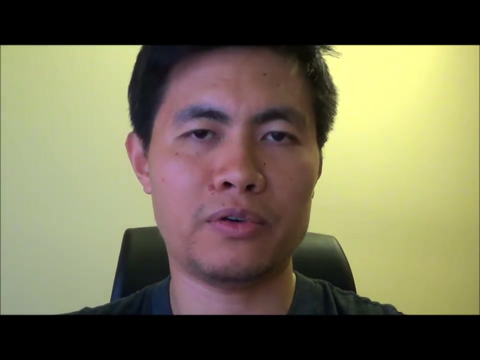 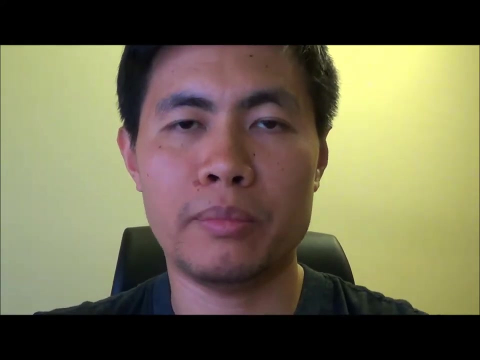 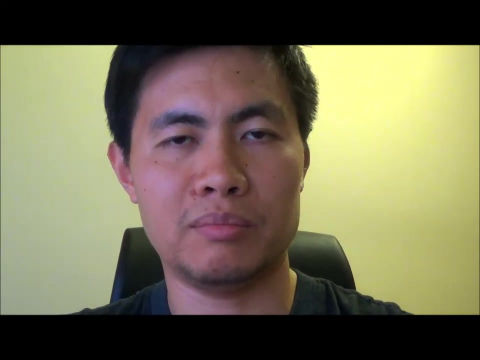 Hi, you're watching Investor Insights and I'm making this video in response to those three or so dozen emails from people that are always asking me or telling me how difficult financial and economic concepts can be and that they're totally overwhelmed. Well, first and foremost, let me tell you that economic or financial systems are actually very simple. 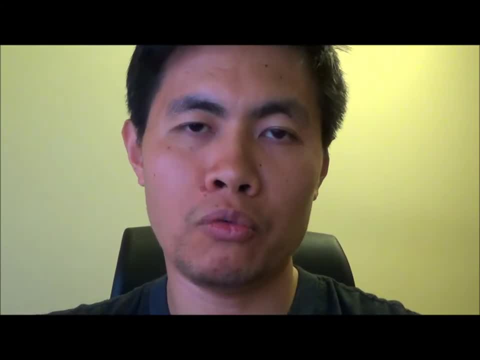 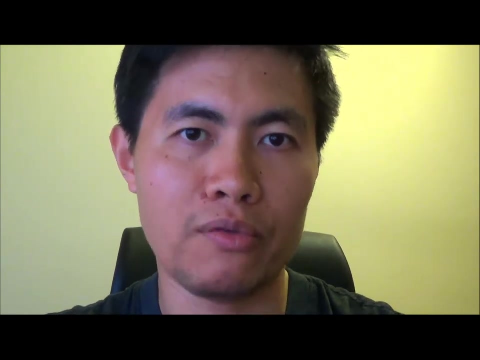 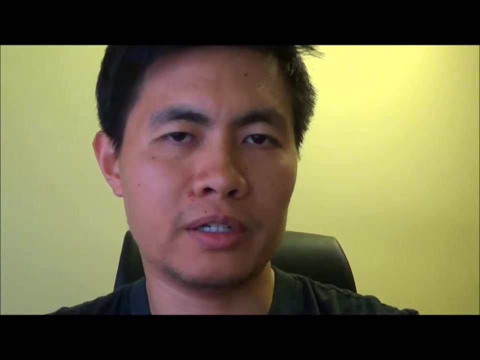 in nature. It's actually uninformed people who want to sound really diligent and intelligent that use big words, such as economists, that make everything sound complicated and thus overwhelming. Just to go off on a little bit of a tangent, if you want to get your head around a very difficult concept, let me introduce you to. 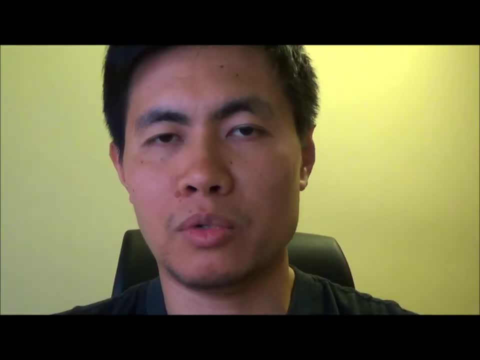 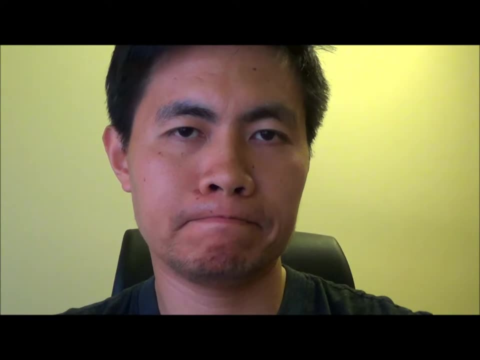 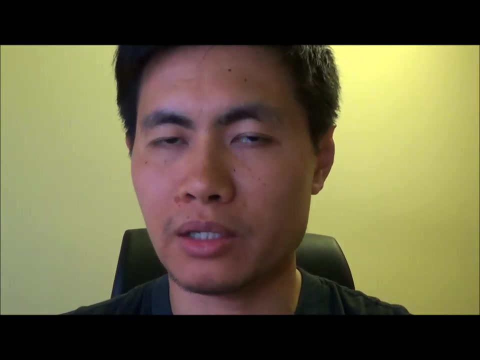 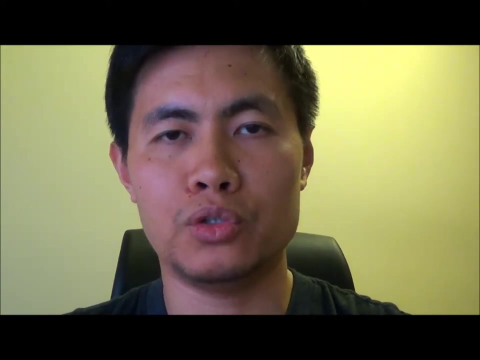 one Now as a cosmologist, everything that has mass we call matter. Now, matter possesses a force called gravity. The larger the mass, the greater the gravity it exerts. So Earth exerts a greater amount of gravity on you than you do on other things. So if you want,